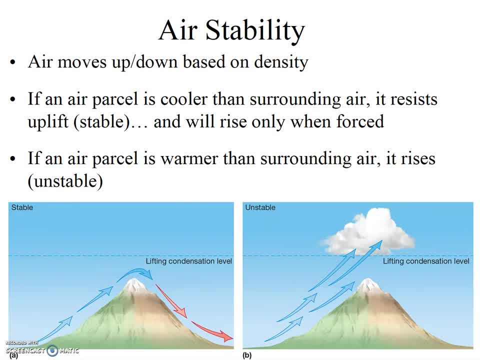 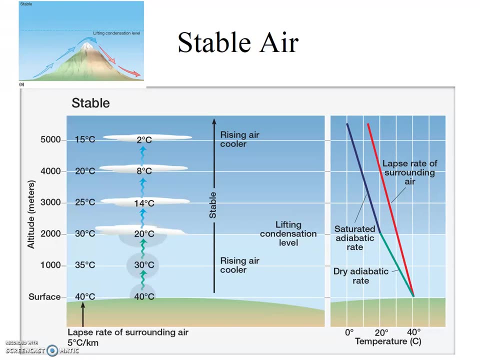 than the air around it. it generally rises, and we call this air unstable because it just continues to rise. We'll look at each of these in a little bit more detail. First, stable air is air that is always colder and thus denser than the surrounding air On the diagram shown here. 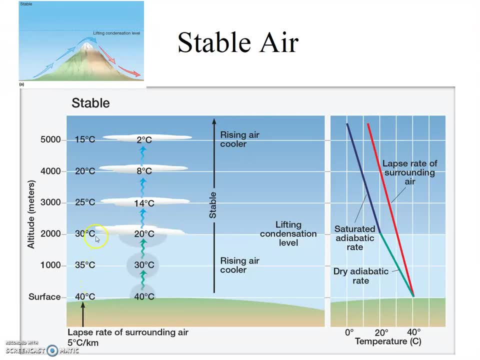 note that they show the lapse rate of the surrounding air. This is just the stagnant air, the air temperature of the air as you go up in altitude, simply because it's further away from the earth, Then over here we have the temperature of the rising and expanding air mass, that is, that is cooling at the dry. 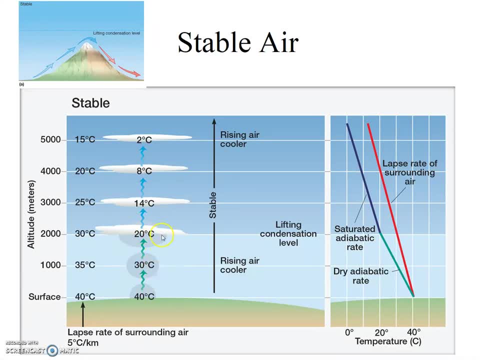 adiabatic lapse rate until the lifting condensation level, and then it's cooling at the saturated adiabatic lapse rate. Notice, in each case here the rising air is cooler than the surrounding air. thus this air will not rise unless it's forced to rise. This is stable air If it's forced to go up over. 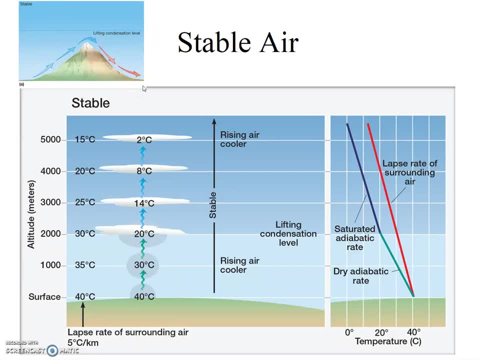 a mountain, it'll come right back down the other side. If we graphed these temperatures and altitudes, we would see the lines looking like this: Here's the line depicting the lapse rate, the environmental lapse rate of the surrounding air, and here the one with: 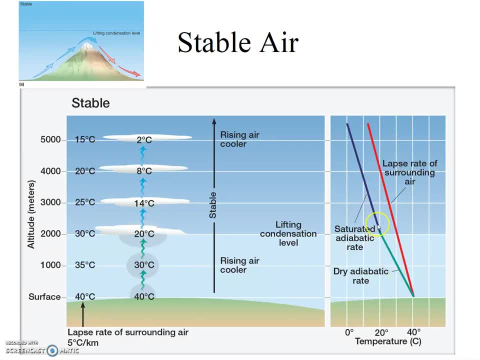 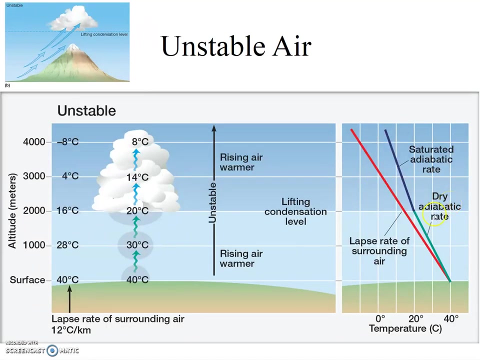 two different slopes representing the DAR and the SAR. we have a line depicting the cooling that occurs as the air mass rises In every situation. here you can see, at every elevation, the rising air is cooler than the surrounding air. Thus this air is stable, Unstable air. on the other hand, when graphed, you can see: 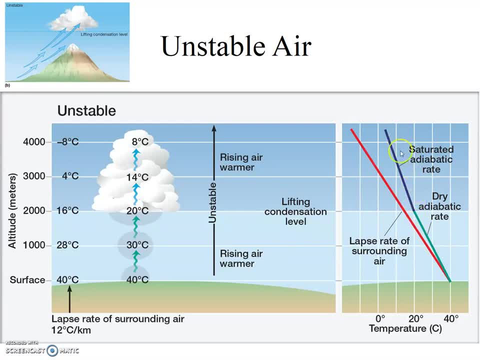 that the the rising air mass. again, the line with two slopes, one depicting the dry rate and one the saturated rate, is always warmer than the the line here depicting the normal environmental lapse rate. You can see that over here as well. Here's the temperature of the stagnant air. 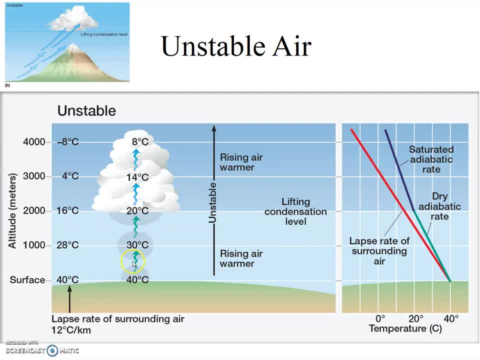 following the environmental lapse rate. and here's this air mass that's rising and expanding. You can see that at every altitude, the rising air is warmer than the surrounding air, so thus it's going to be less dense and we're going to expect it to continue to rise. You can see that in this diagram, here, In fact. 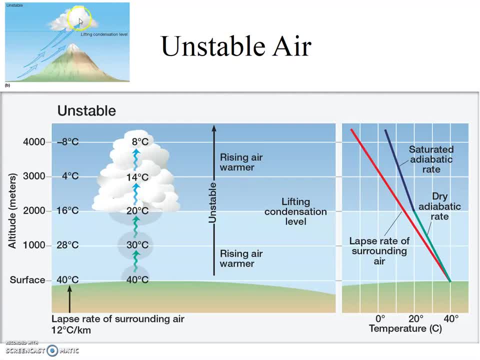 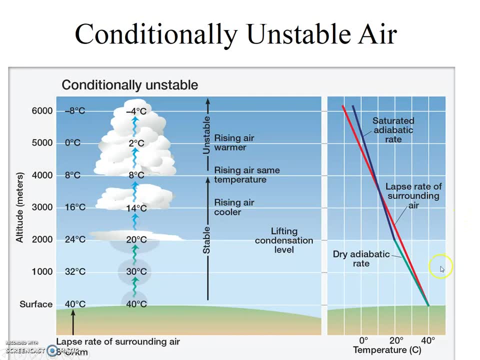 that the air has risen enough that it's become completely saturated and formed a cloud in this diagram. Check out this third case: conditionally unstable air. Can you figure out where the air would be stable and where it would be unstable just based on this graph here? Pause the video for a moment. 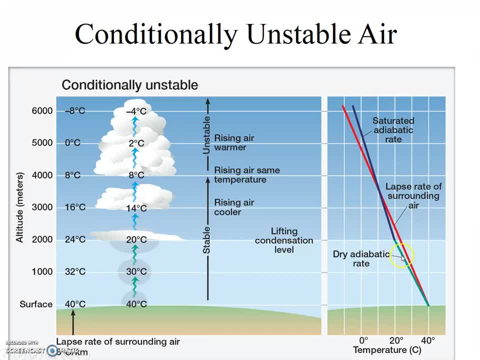 Hopefully you were able to see that anywhere that the temperature of the rising air is cooler than the surrounding air, it's going to be stable. It's not going to want to rise. On the other hand, up here further, the temperature of the rising air is warmer than the surrounding air, so this: 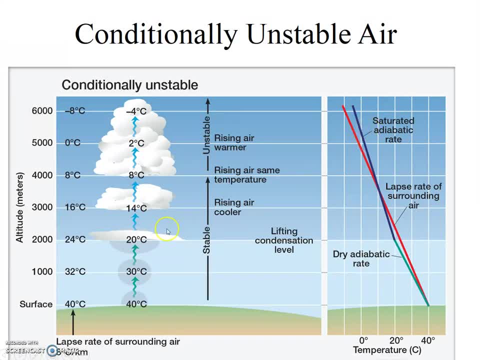 would be unstable air that would be rising. So in this case, if this air got pushed up high enough due to some sort of uplift that we haven't talked about yet, if it got pushed up high enough, it would then start to rise spontaneously on. 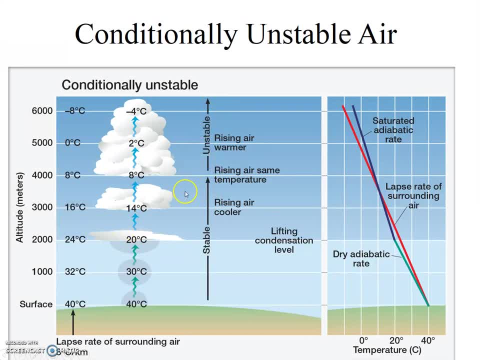 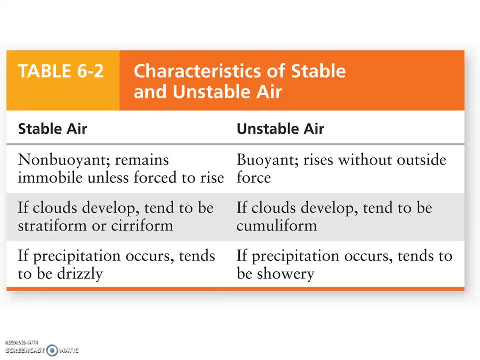 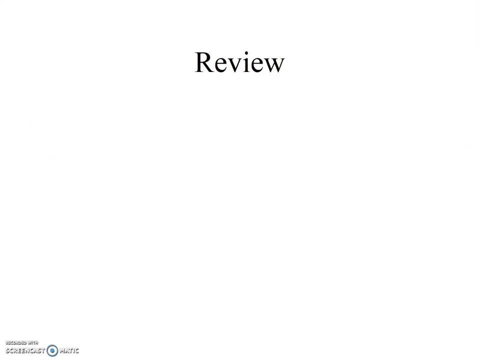 its own and be unstable. If it never reached that point, it would simply fall down again if left to its own devices. Table 6.2 gives a synopsis of the characteristics of stable and unstable air. Pause the video, check it out. So let's review a few important concepts in 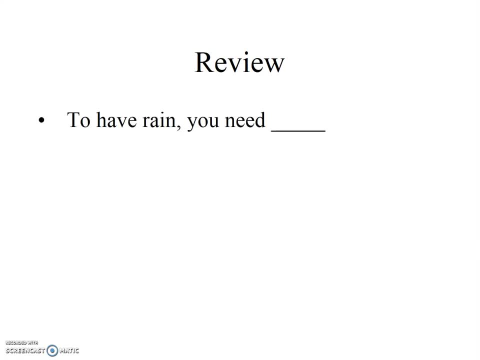 the last several video clips. First of all, to have rain, you need clouds, and to have clouds, you need water. you need what? What two things are needed in order for condensation to occur? Hopefully you said saturated air and a surface for condensation to occur on.